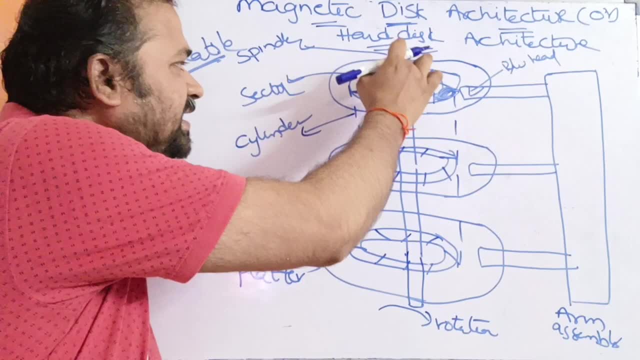 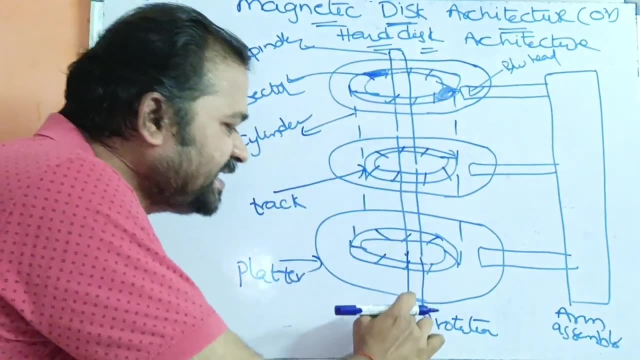 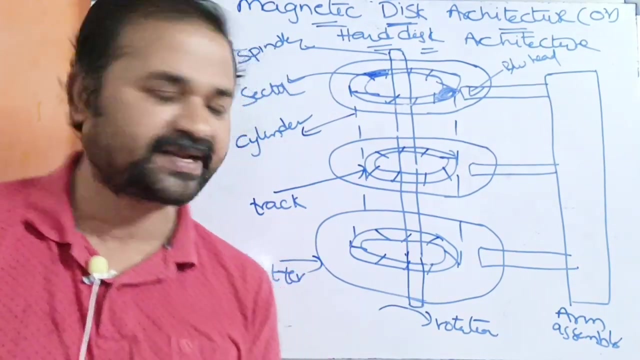 like CD Next year. platters are connected together with the help of the spindle, So this is called as spindle. So spindle is mainly useful in order to connect all the platters together. Here we can rotate the spindle. If we rotate the spindle we can see that the platter is connected to the 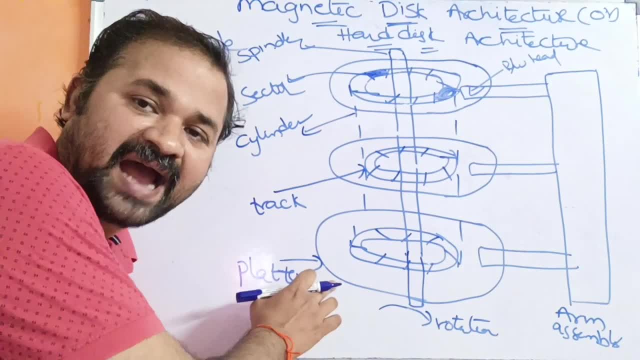 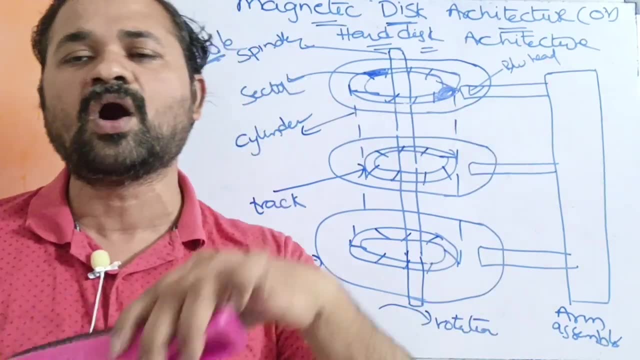 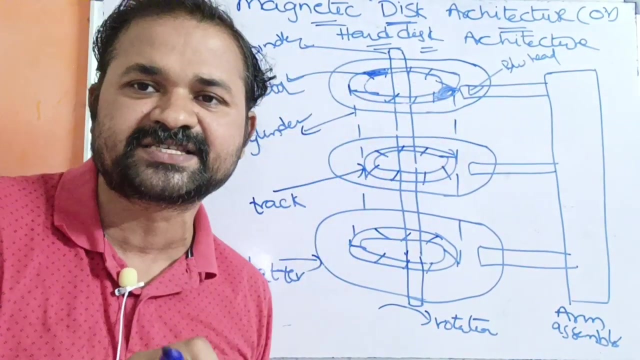 spindle. So if we rotate the spindle, then automatically the platters will be rotated. We can rotate the platters either in clockwise direction or anti-clockwise direction. Next, here we will have two surfaces on each platter, So this surface is called as top surface and 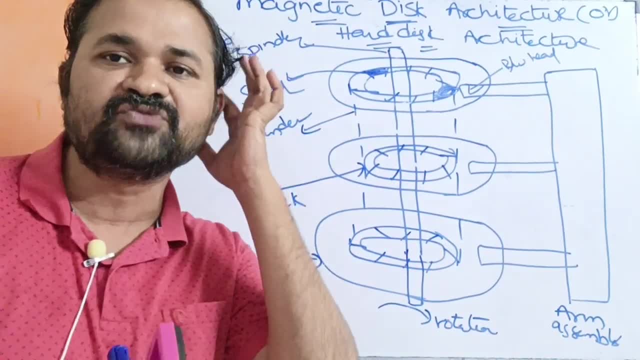 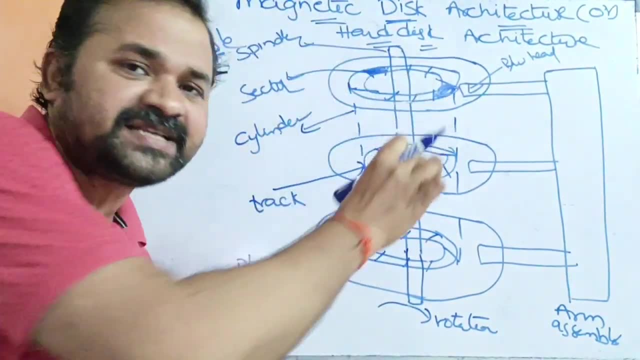 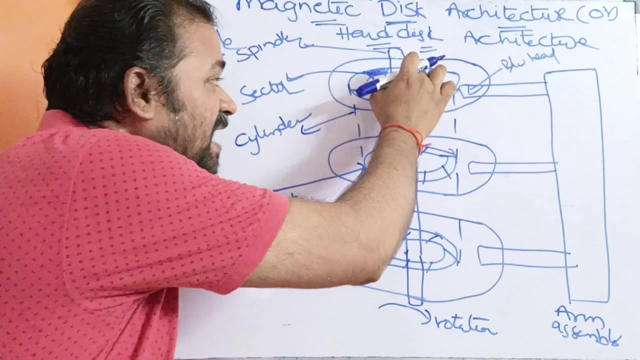 this surface is called as bottom surface, So we will have two surfaces on each platter. Next point is platters are subdivided into tracks Here. this is a platter, So we can divide this platter into a number of tracks. So this is one track. This is another track, So this is second. 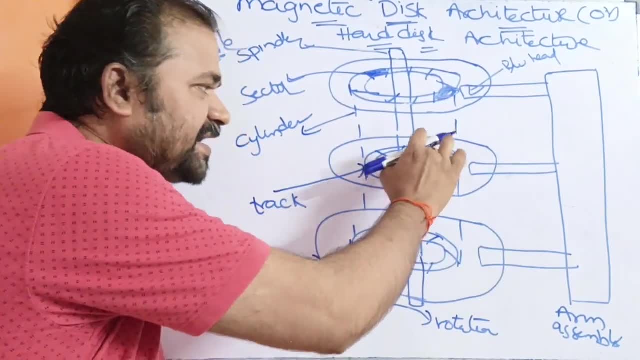 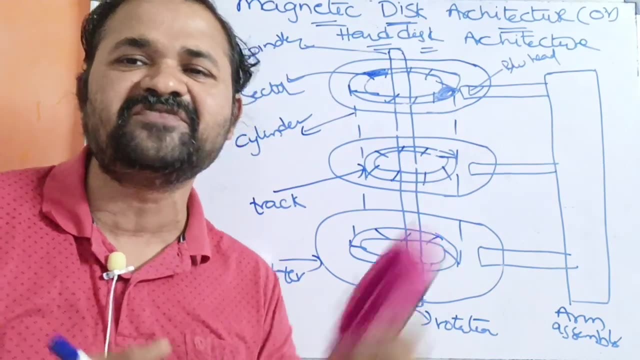 platter. So this platter is divided into a number of tracks: Track 1, track 2.. This is a platter. This platter is divided into two tracks: Track 1, track 2.. So likewise, we can divide the platters. 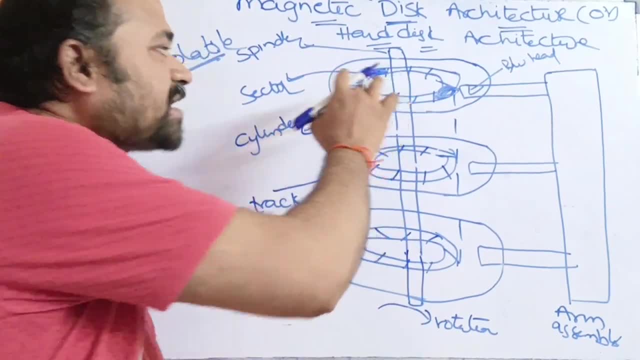 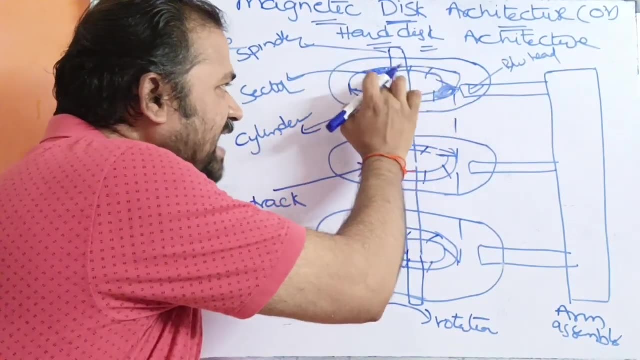 into two tracks. So we can divide the platters into two tracks. So again, the tracks are subdivided into various parts, called sectors. Here this is a track, This track is divided into several sectors. So this is one sector, This is another sector, This is third sector. 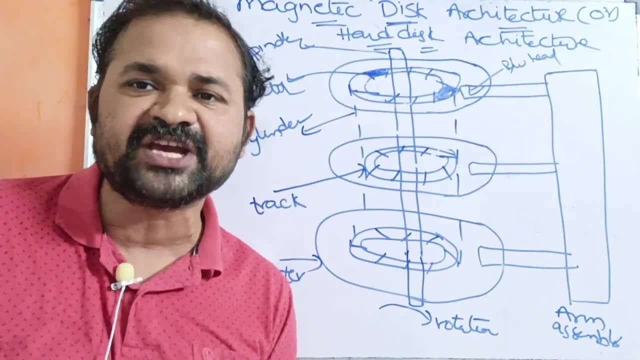 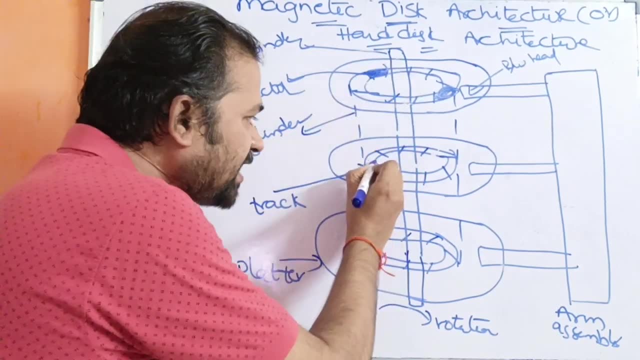 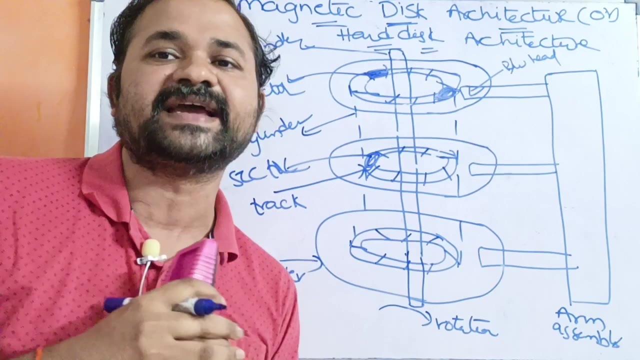 Next to sector. likewise, Here the information is mainly stored in sector. The data will be stored in sector. So this is one sector. So likewise, this is another sector, Another sector, So the data will be stored in the sector. The number of sectors in each track. 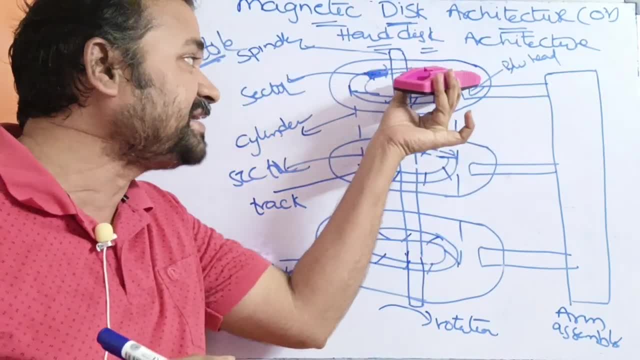 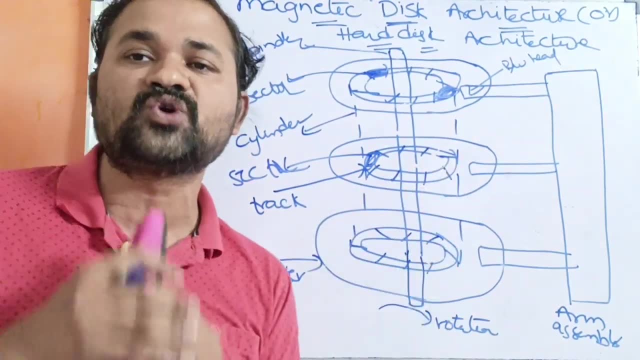 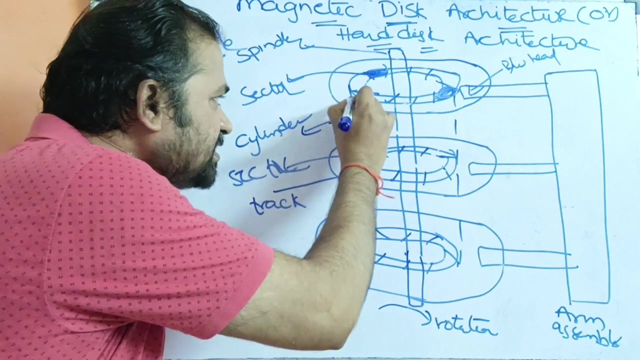 must be equal. So let this track contains 256 sectors, Then this track, as well as this track, should also contain 256 sectors. And the next point is: here we have cylinder, So this portion is called a cylinder. Okay, The set of tracks.